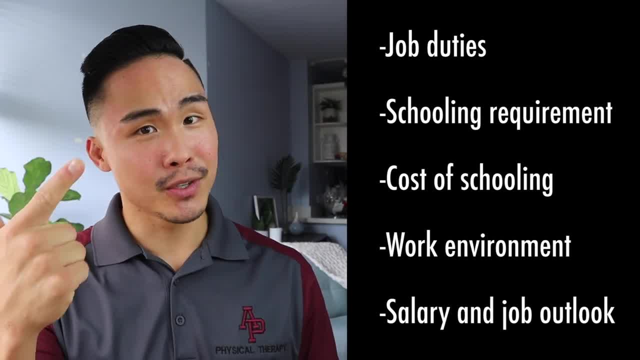 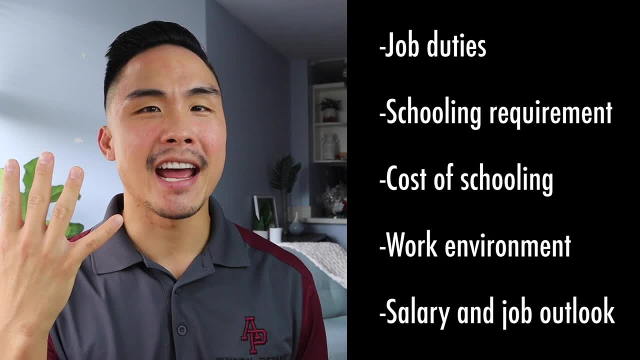 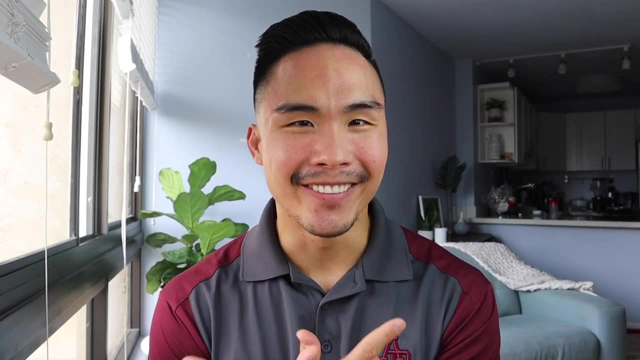 physical therapy. physical therapy: The last three categories we're going to talk about are job duties: the amount of schooling it's going to take, the cost of schooling, the work environments and the salary and job outlook for the next 10 years in each profession. So let's just get into this lego. 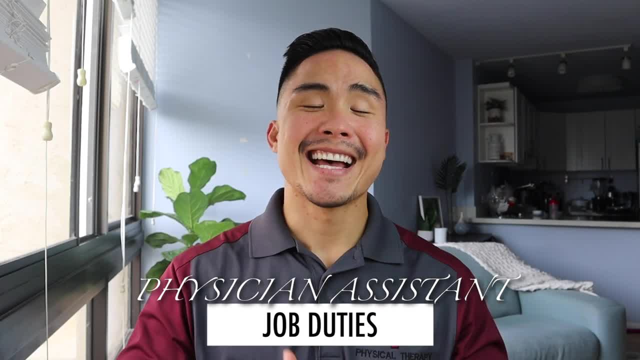 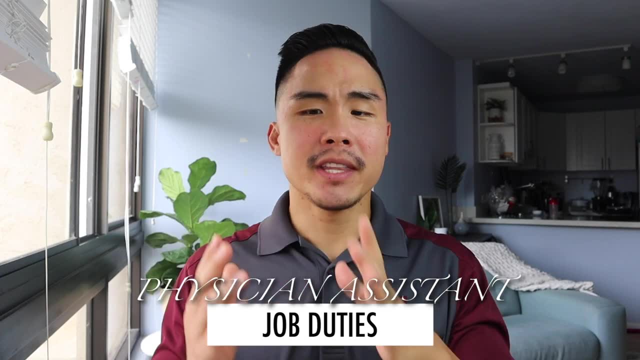 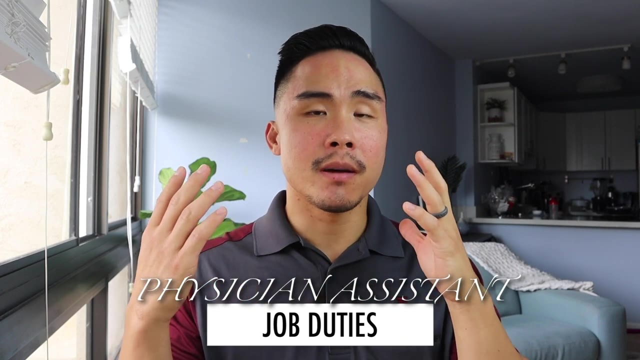 All right, so job duties as a PA, as a physician assistant, you are pretty independent. now I know the name physician assistant makes it sound like you're an assistant. but physician assistants, these, these, uh, this profession is pretty independent in what they can do. they can diagnose, they can treat, they can do. 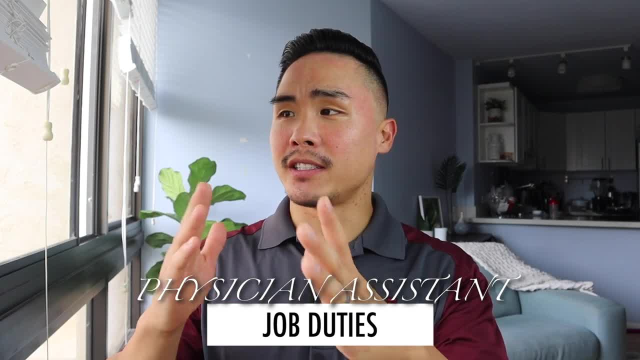 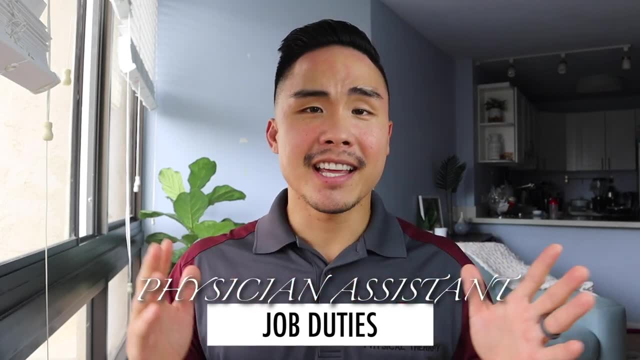 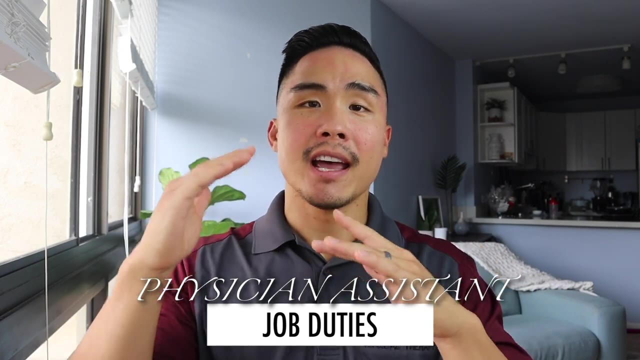 lab tests, they can give x-rays, they can uh differentiate and refer patients to different, different, uh different- healthcare professions, and if there's anything that's not within their scope of practice, then of course they can go to their supervisor or their higher-up physician and get a sign off as to, maybe, which medication they can administer if it's not within their 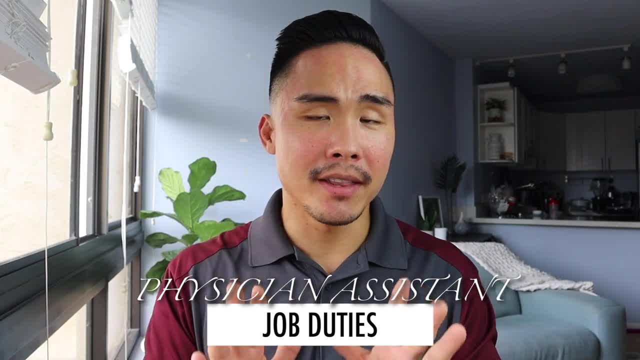 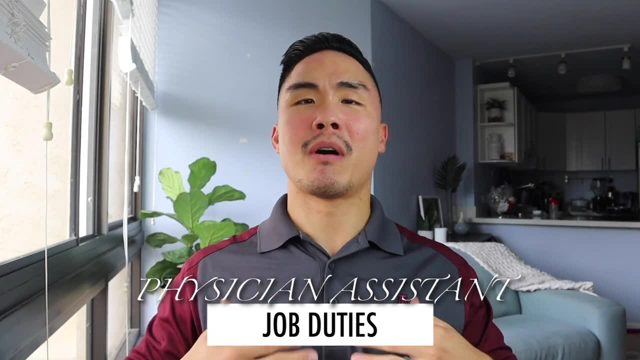 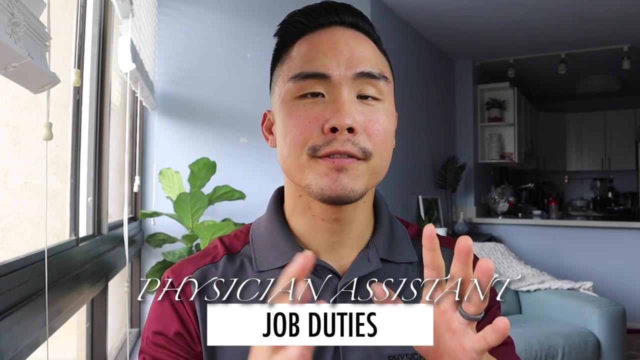 scope of practice. so there's a ton of independence with this career and I just want to let you know that up front because I know the assistant might make it sound like, oh, I'm not the top dog kind of thing, But there's actually a lot of things that PAs can do. So just to give you a general 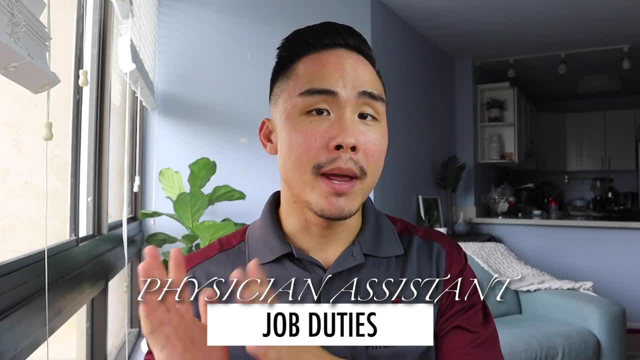 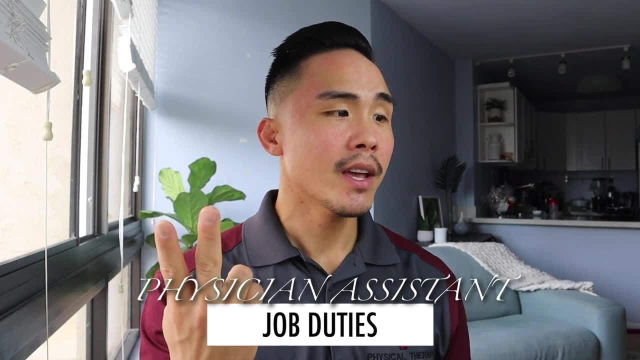 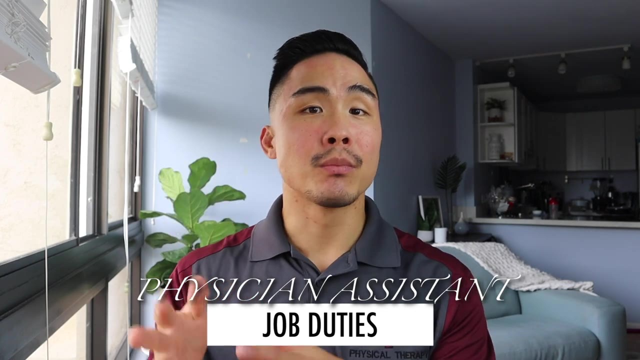 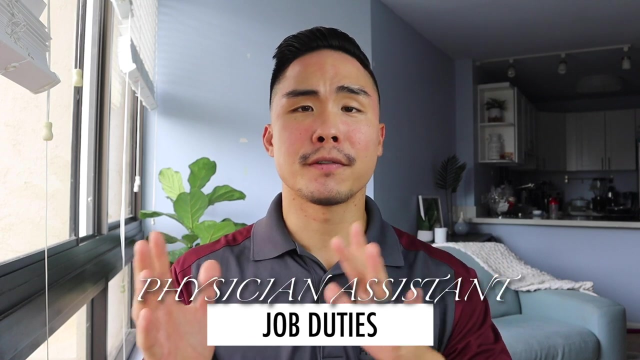 description of what PAs can do. They also make rounds right in the hospital. They perform different exams to evaluate and diagnose them. They are able to prescribe and administer medication. They can order and interpret lab results like blood tests or different other tests and x-rays. They can definitely refer them to different health care providers for whatever might be best for the patient. 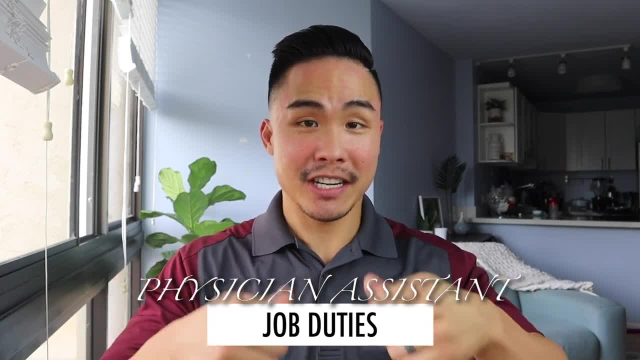 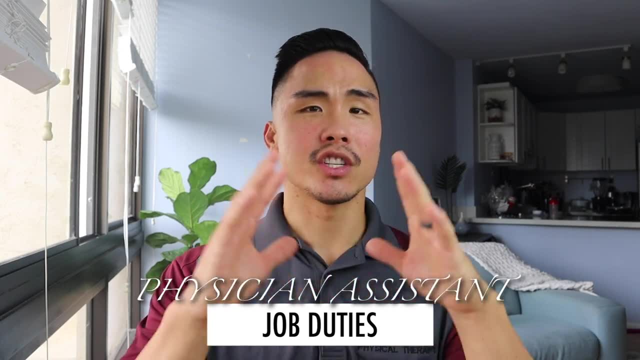 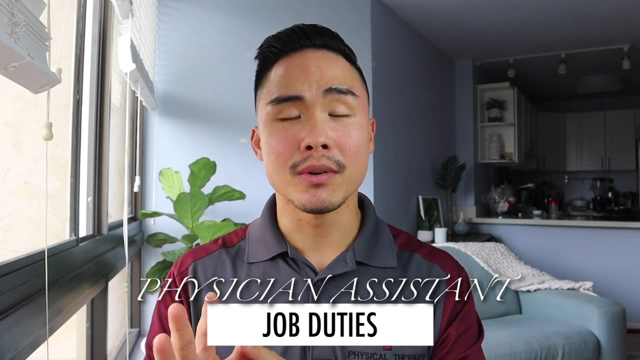 And they can assist in surgery and they can actually go in and do some stuff with their own hands, Which is really, really neat. Now, of course, this is a general job- duties that physicians can do, But I just want to let you know that they are super independent in what they can do. 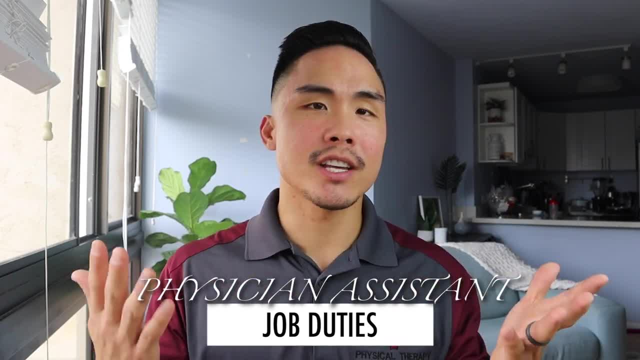 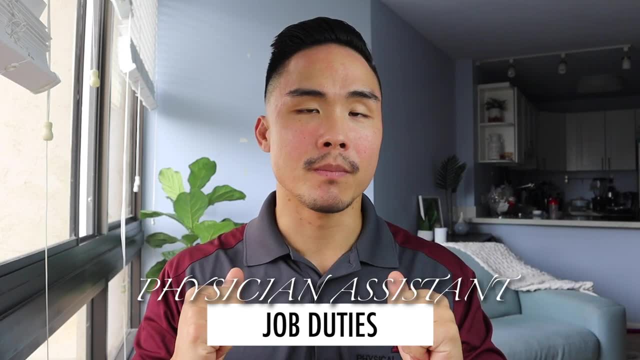 And if it is not within their scope of practice, then they just ask their supervising Physician to sign off on whatever they may think. and if the physician signs off, then boom, there you go. So, for example, if a patient might need a certain medication, 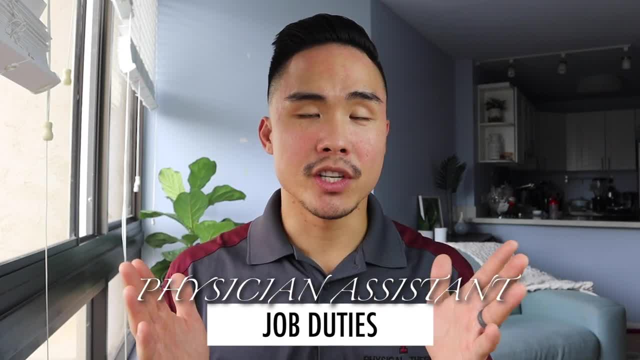 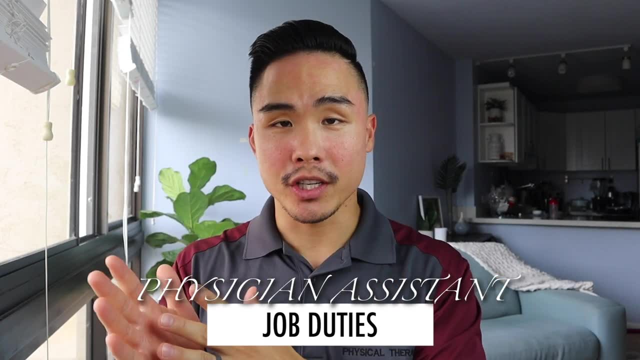 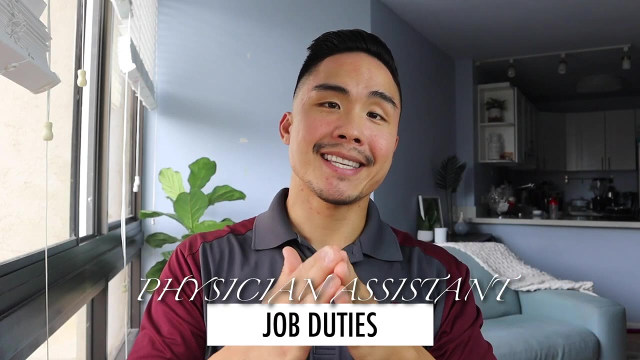 Let's just call this medicine A, and it's not within the physician scope of practice, But they think that it's. they think it is. it is appropriate for the patient. Then what they'll do is they'll ask their supervising physician: Hey, can I give patient medicine A? because of these different things? 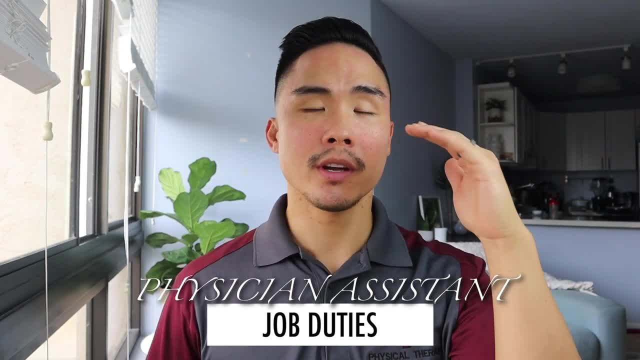 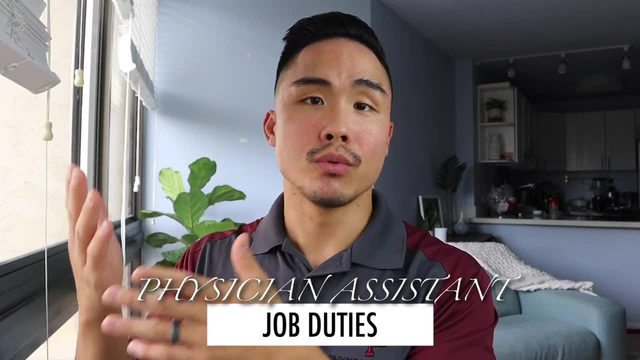 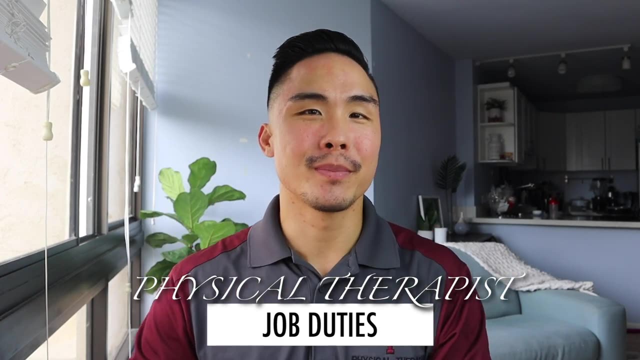 And if the physician says, hey, you know what, I think that is appropriate, then they'll sign off on it, And then then the hospital gets the orders that the physician can give this type of medication to the patient. All right Now, physical therapists: you guys know a lot about what we do already, because this channel is all about physical therapy. 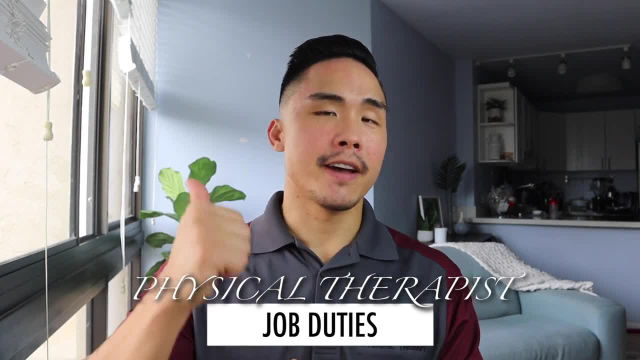 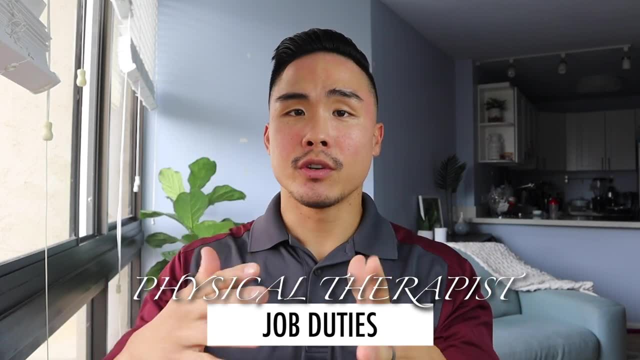 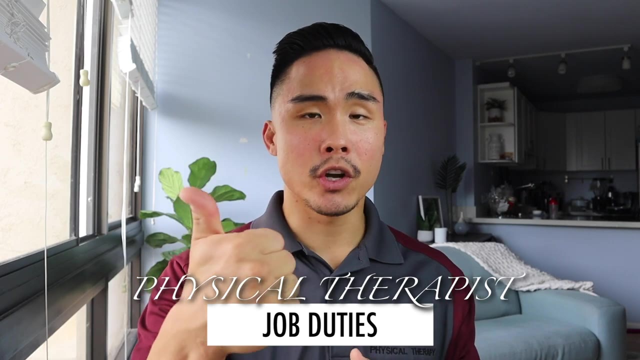 But just as a quick review. Physical therapists can evaluate and diagnose different movement disorders and help optimize human movement. our treatments We can do for patients are to help them return to their prior level of function, and different treatment options might be like manual therapy, therapeutic exercise, therapeutic activity, gait training and 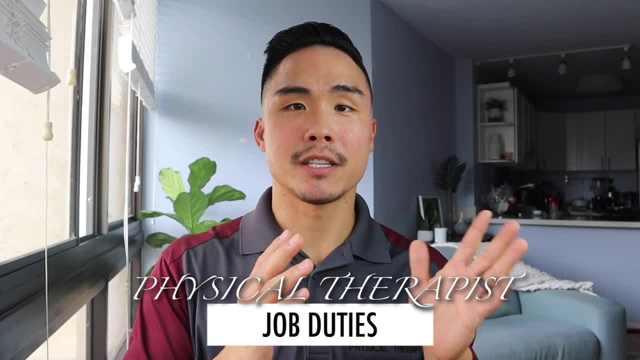 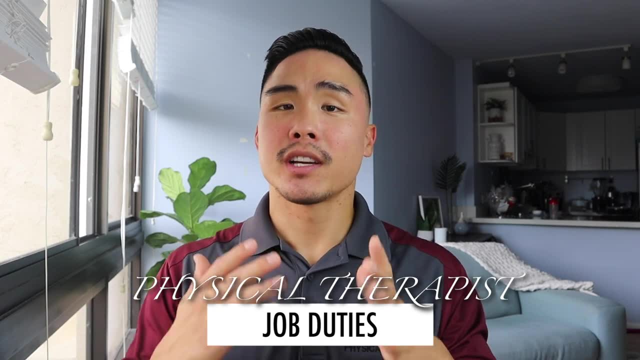 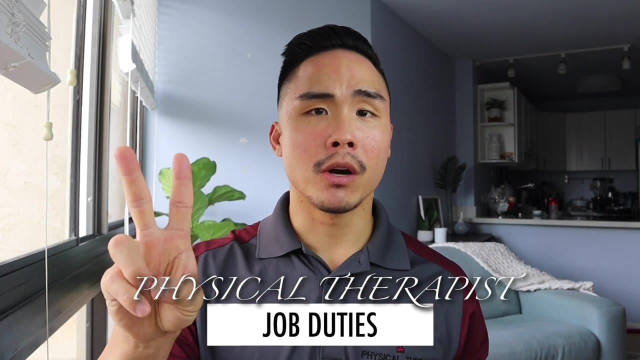 neuromuscular re-education and we can use different modalities and special scientific agents like ultrasound, mechanical traction and things like that. we also can help fit and evaluate a patient for different assistive devices like wheelchairs, power wheelchairs, electric scooters. 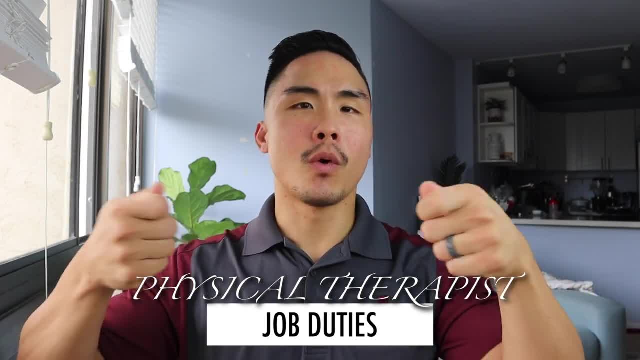 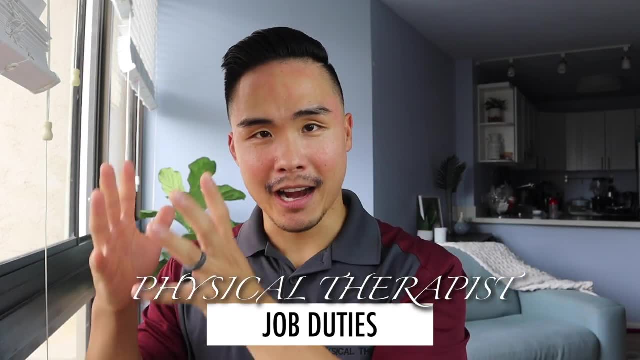 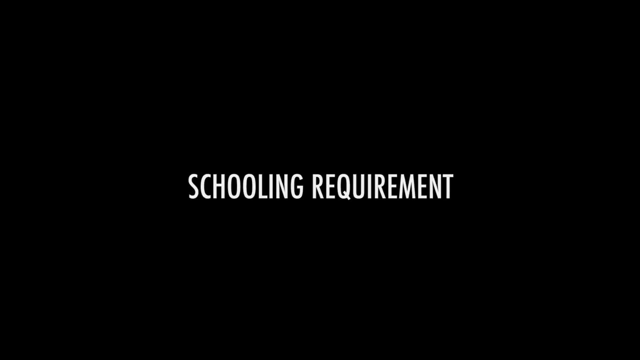 axillary crutches, four-wheel walkers, different types of canes, things like that, and ultimately, our goal is to help a patient go from where they are at and help them return to their prior level of Function so that they don't need our services anymore. Okay, schooling guys. 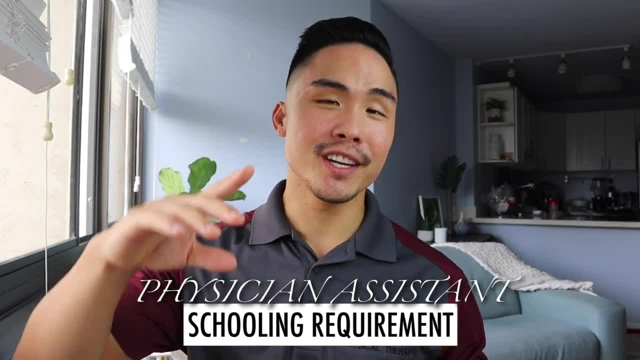 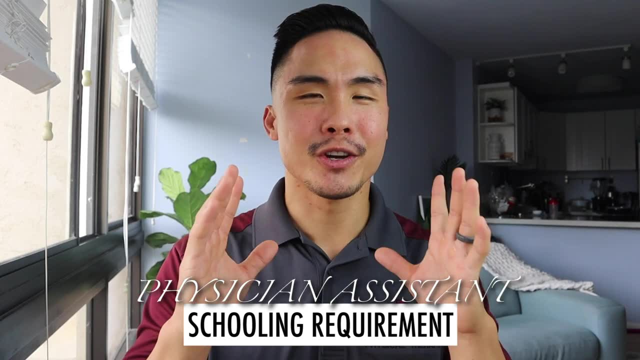 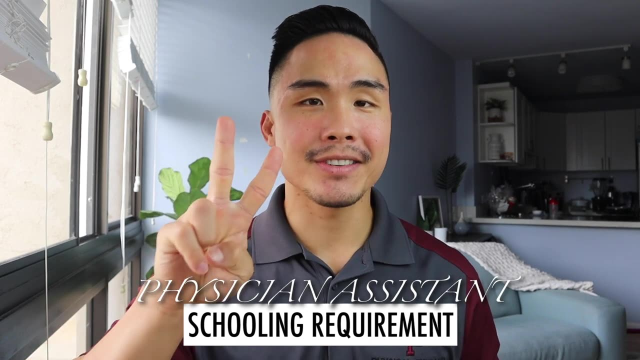 This is gonna be crazy for you because the amount of schooling, the cost and the salary for our different professions is Gonna be really eye-opening. So make sure you're paying attention. so schooling PAs require only two years for a Master's degree and they have to sit in for a licensing exam to work as a PA. 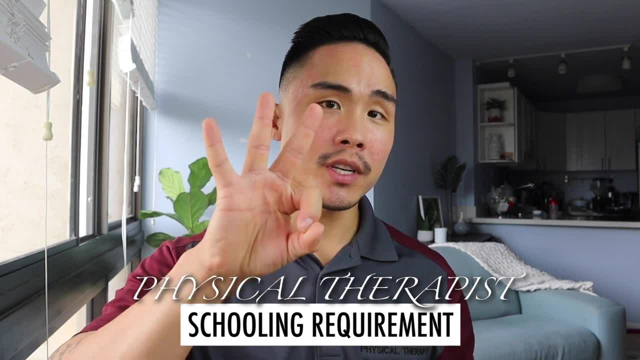 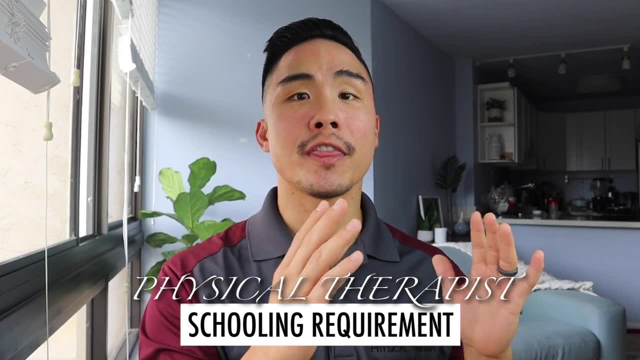 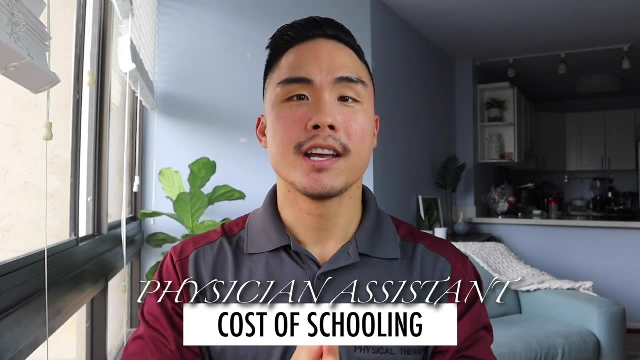 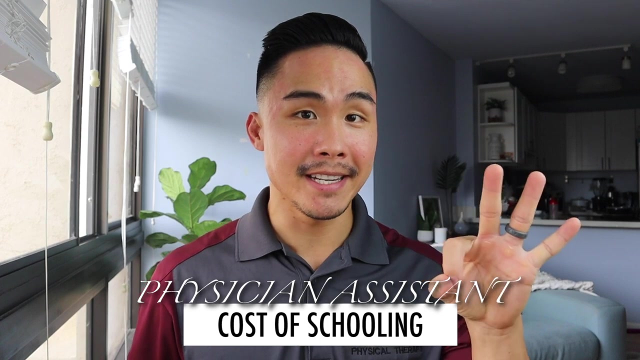 For a physical therapist, you need to be in school for three years for a doctorate degree and then you have to sit in for a licensing exam to work as a physical therapist. All right, so let's talk about cost now. Remember I talked about the schooling: two years masters for PA and three years doctorate for PT. 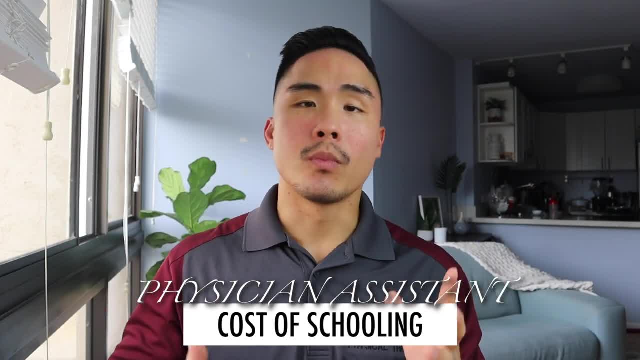 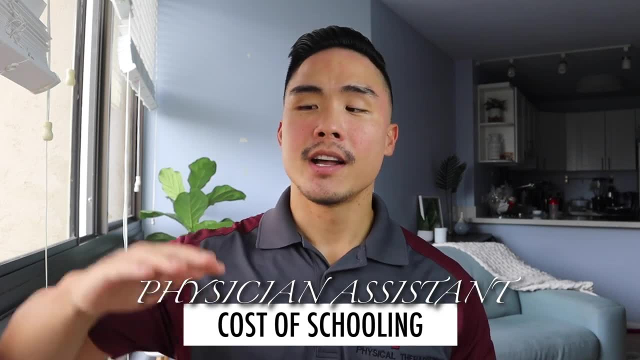 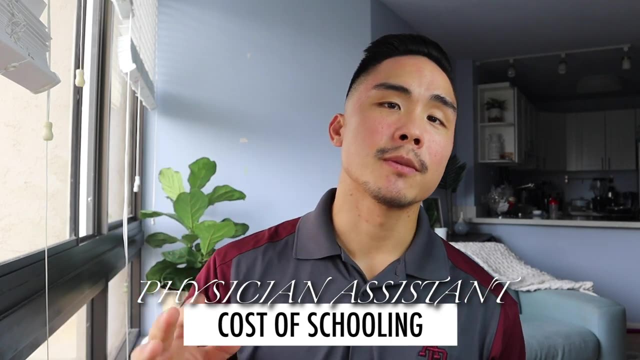 But the cost is gonna be different, Of course, when it's private versus public, and if you're a resident or not. All right, So let me give you some details. now, when we're talking about physicians, assistant PA, if you're a public resident, your tuition will cost about 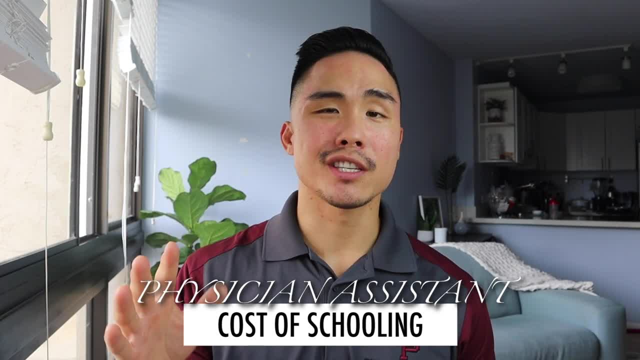 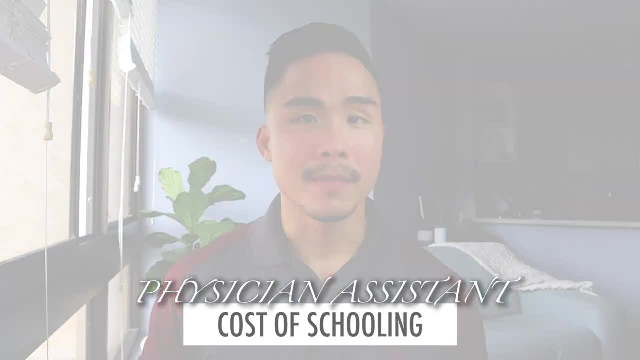 $50,000. if you're a public non-resident will cost about $88,000 and if you're in a private institution will cost about $90,000. now for a physical therapist you have a variety of course for public and private, but on average 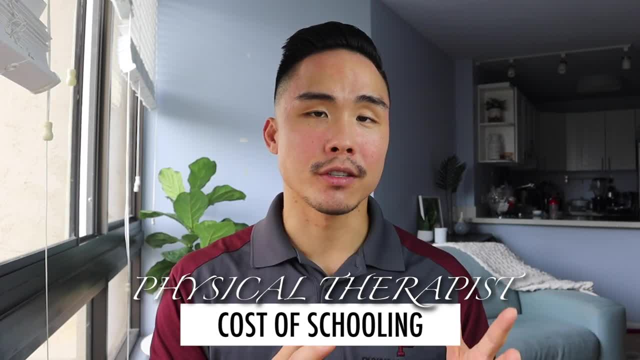 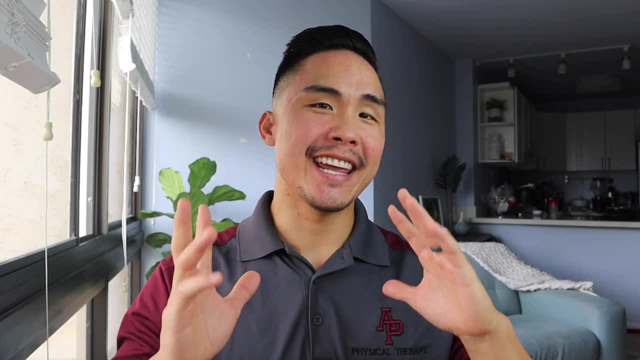 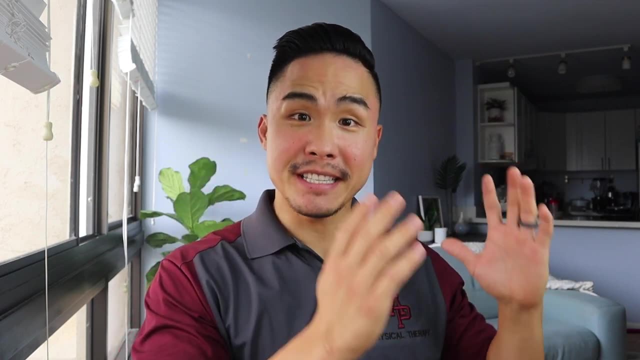 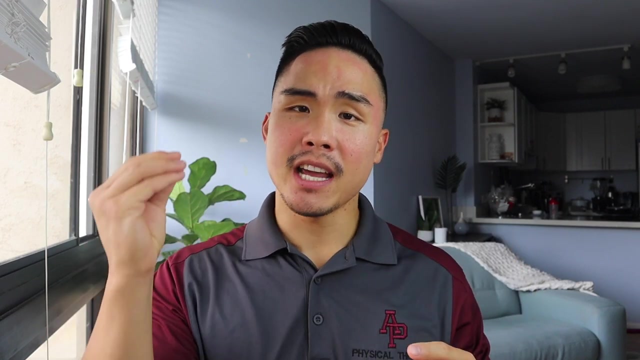 It's gonna cost about a hundred and ten thousand dollars for tuition alone. All right, so let's talk about work environment Now. PAs can work in a variety of fields along with PTs as well, And a lot of times these two professions will work hand-in-hand with each other. if a PA finds that hey. 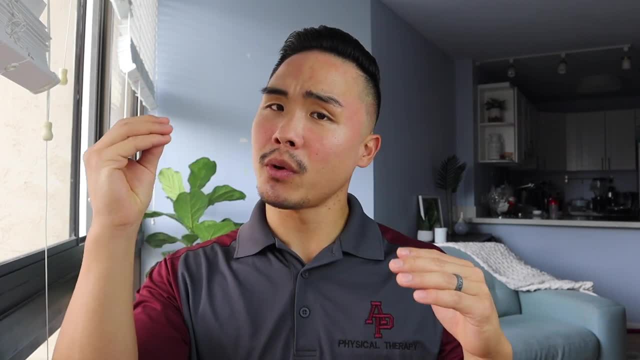 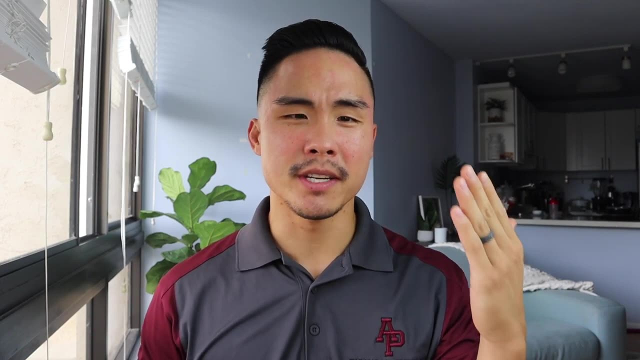 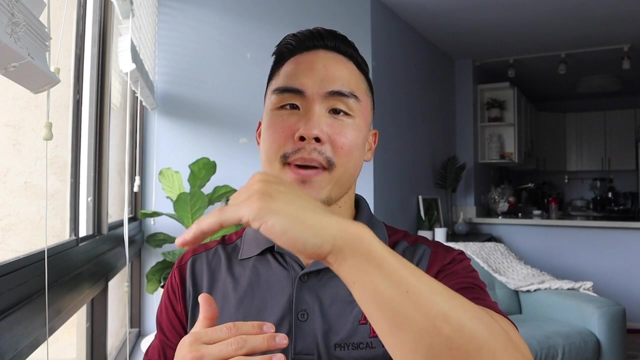 You know what you might benefit from physical therapy a lot down there- refer them to the physical therapist. and a physical therapist Might get a patient and say: you know what, you're not appropriate for PT. You should go back to see your, your primary care physician, Or maybe you're a physician's assistant. then they refer them back to the physician's assistant or the physician. 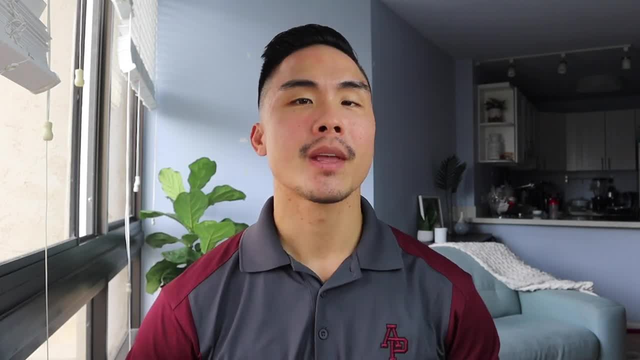 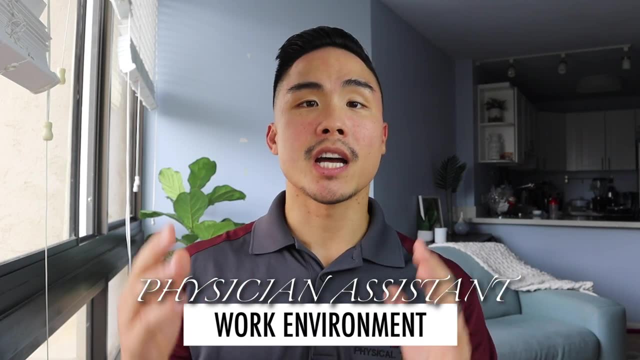 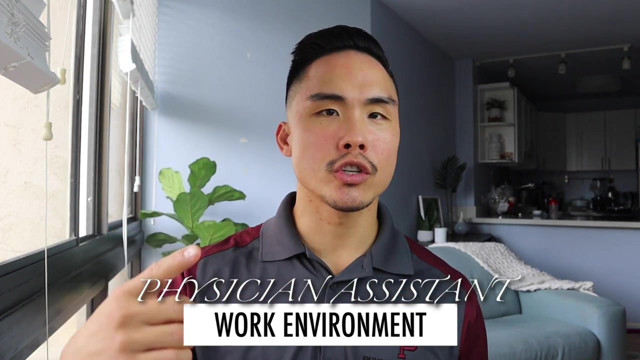 Which is where the physician assistant will work under now work environment. physician assistants can work in many different fields, but most of the times they will be working in a Hospital. now, in the hospital- of course they're in different floors- They can be in surgery. 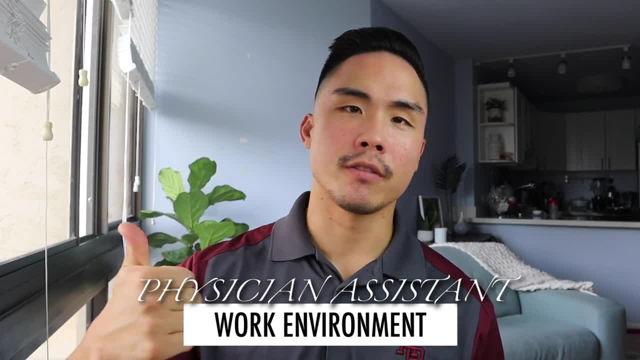 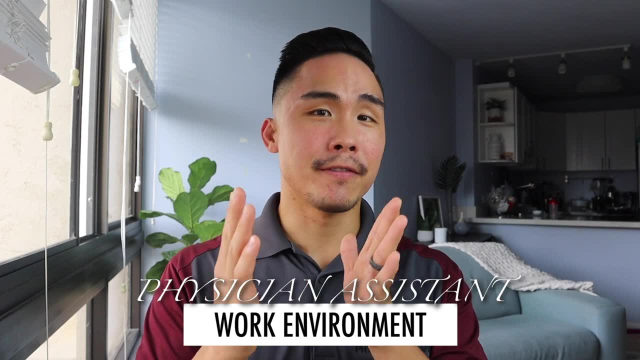 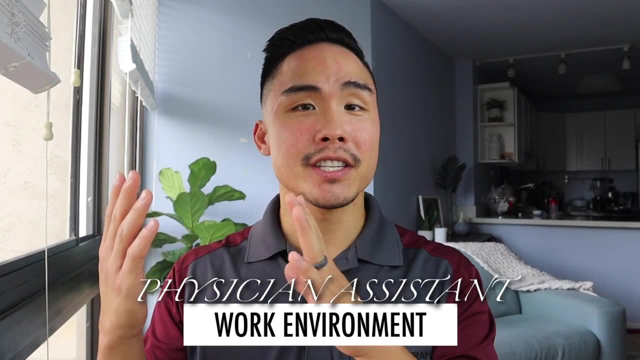 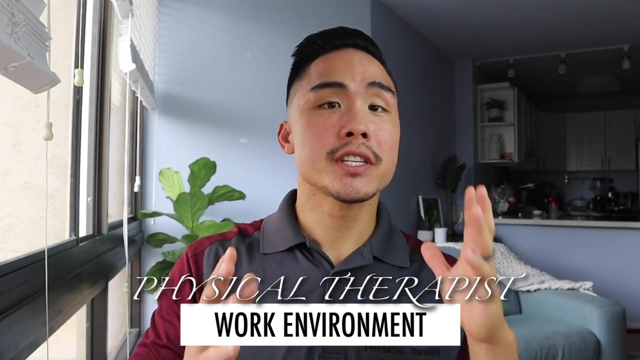 emergency department on stable floors. orthopedics, cardiovascular, neuro, all of those different things. they can also be working in outpatient offices, like under a physician, in a physician's office, and They can also be working in different centers like convalescent homes, Skilled nursing facilities and things like that. Now, a physical therapists are very similar as well, right? 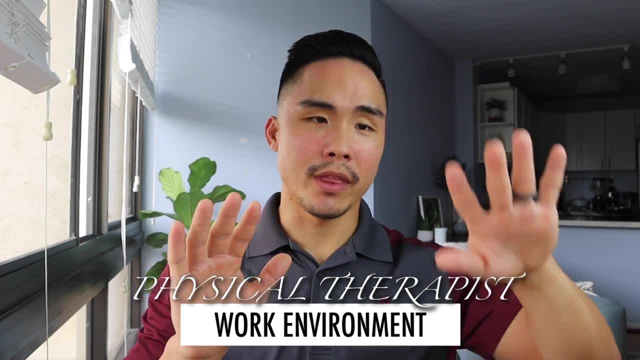 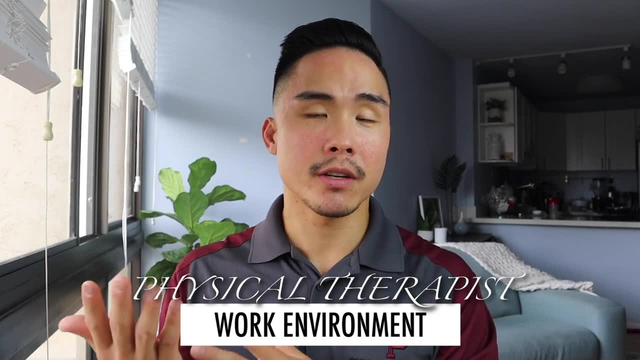 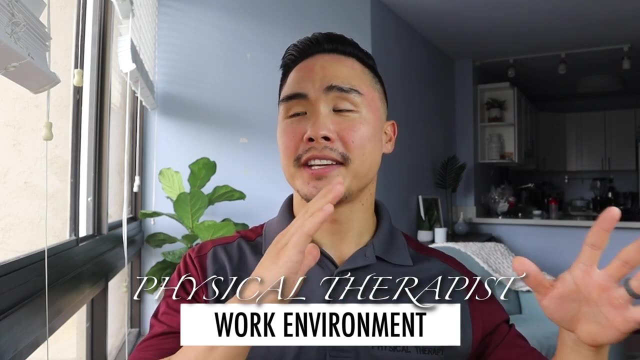 Typically there are two different categories: You're being the inpatient or the outpatient, setting in the inpatient You're either working in the hospital or like a Skilled nursing facility or convalescent home, and then in the outpatient, You're typically working in the outside world where patients are a little bit more stable and in different specializations, right. 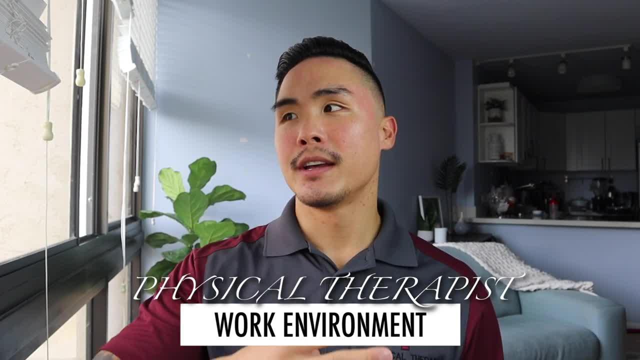 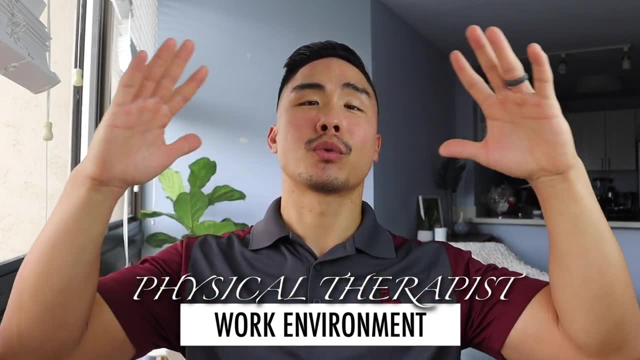 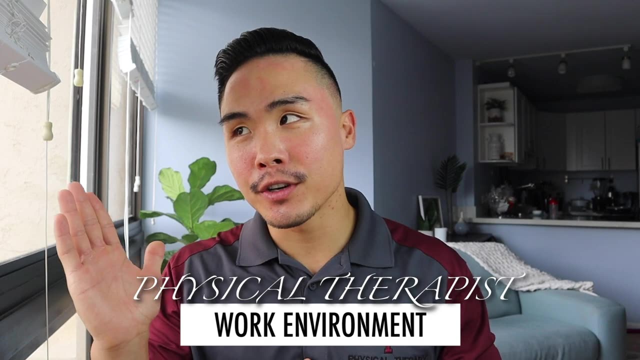 So you have orthopedics, neuro pediatrics, aquatics therapy, Hippotherapy and so much more. so both professions work in a variety of different clinical settings. So if you're really up for hey, you know what I want to work in this place first, and then maybe I'll get. 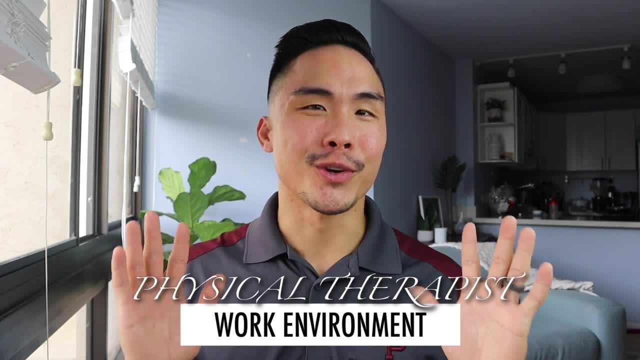 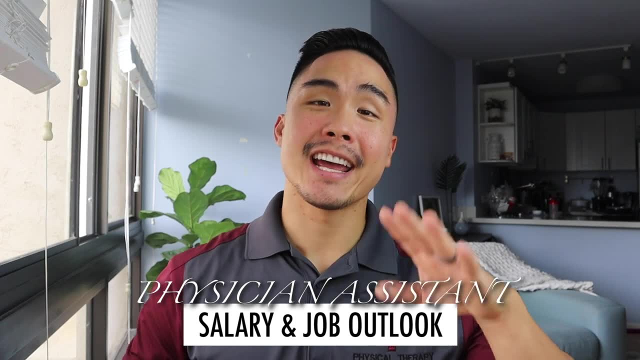 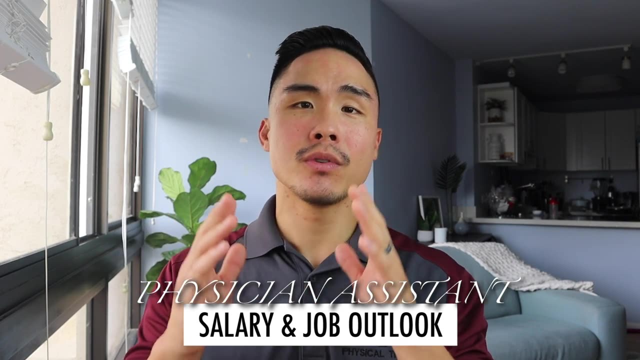 Tired of that and I want to work in this place. both professions are great for that. All right, let's talk about salary and job outlook. now I got this information from the Bureau of Labor Statistics, which will give the annual and median salary for the next 10 years, from 2019 to. 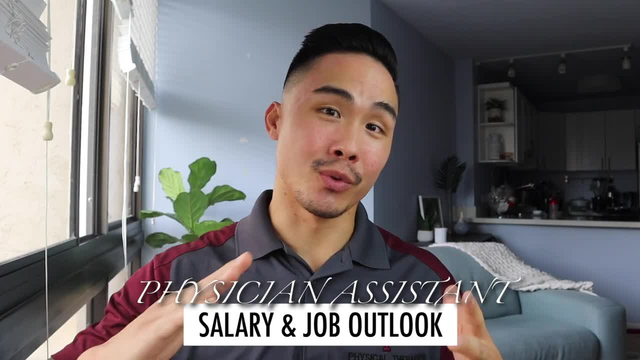 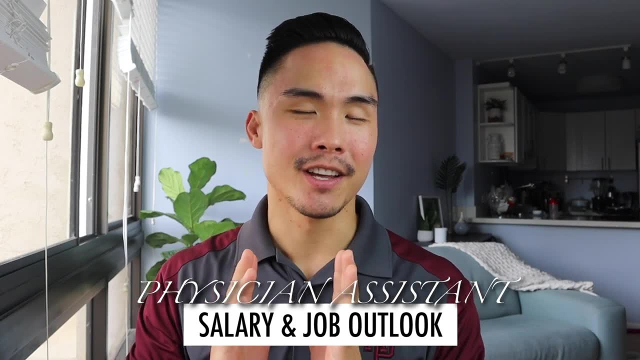 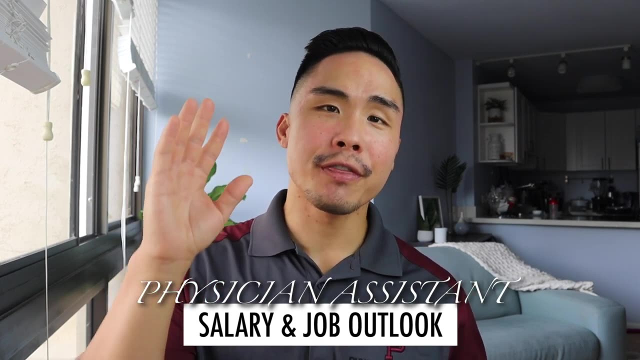 2029 and the job outlook, whether it's gonna grow or not grow and at what percent. right, So check this out. This is actually super great information for you guys. so a physician assistant: the average salary is gonna be a hundred and twelve thousand dollars a year, and 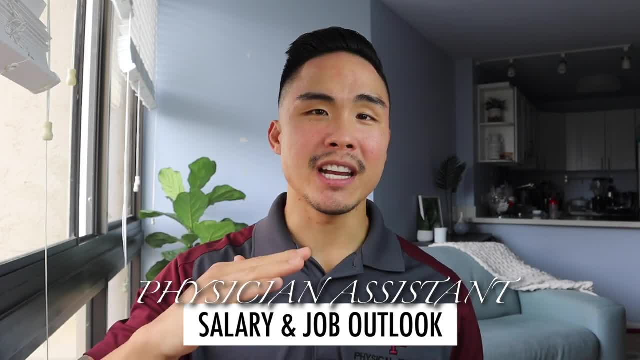 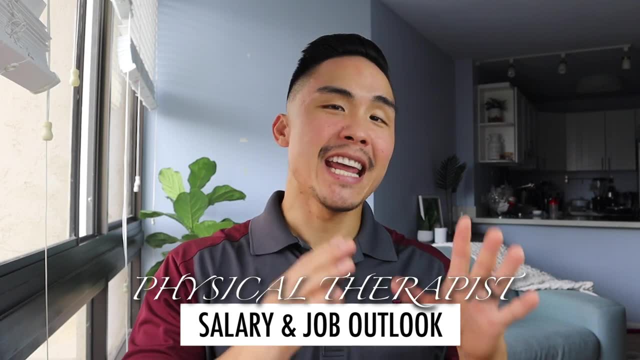 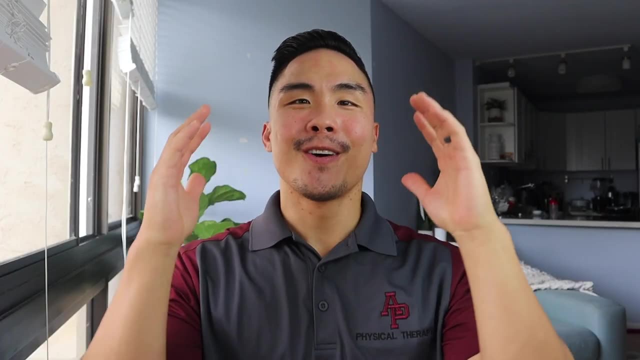 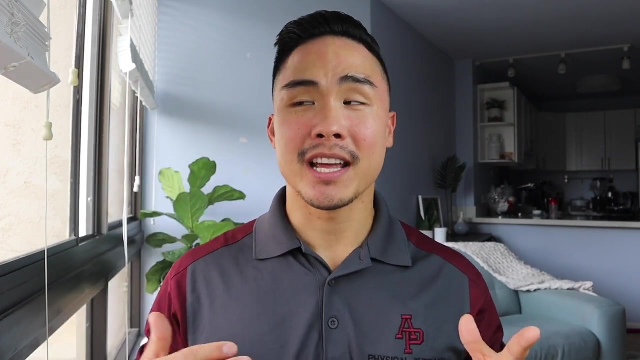 The job outlook will grow at a rate of thirty one percent. now a physical therapist. the average salary will be $89,000 a year and the growth will be at 18 percent. All right, so you guys. learn the differences between PA and PT and the different categories that you might really want to consider when you're choosing the different professions. 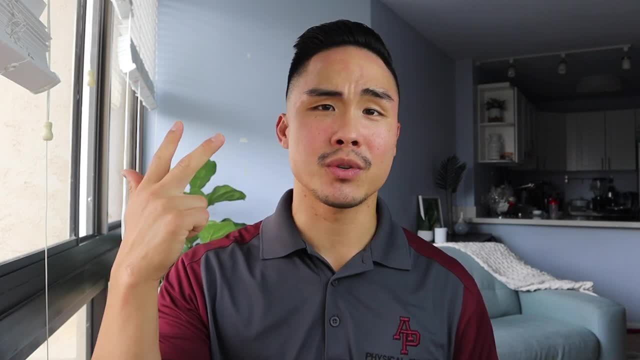 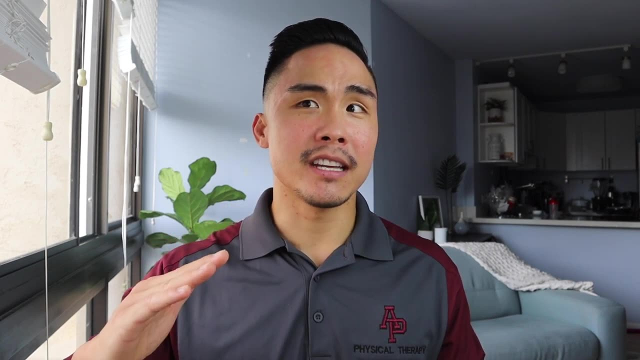 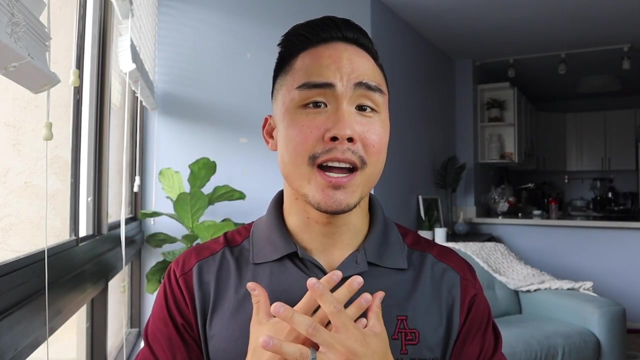 Whether that's their job duties, their work environment, the cost of schooling, the amount of schooling and the amount of money You're gonna make after and, really importantly, is the job gonna grow or is it gonna start plateauing out now? considering these things, in my opinion, guys, PA versus PT. PA is gonna be super beneficial in the future, Like and me as a working physical therapist. if I had to go back and if I was about Money and and if I was okay working in the hospital and administering medicine, practicing medicine, Heck yeah, I would become a PA for the amount of schooling that you need, for the amount of tuition that it costs. 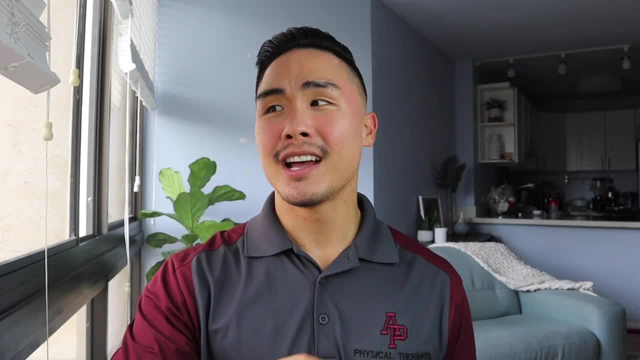 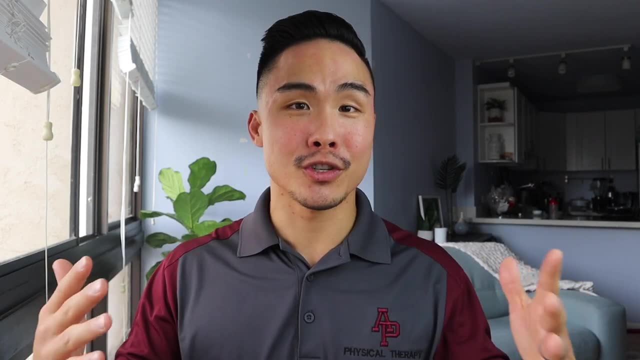 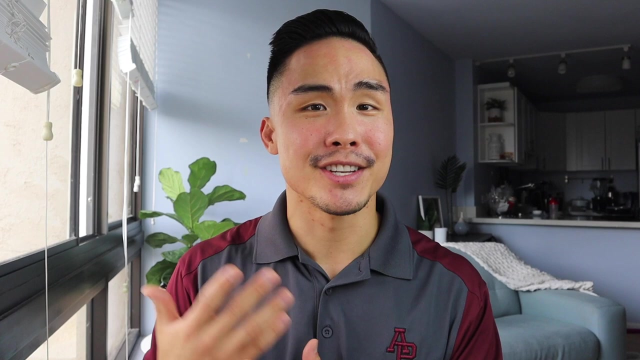 And the amount of money you're gonna make and the job outlook. man, I'm gonna always have a job. There is so much security in this and I'm gonna be making a lucrative future. have a lucrative future For the amount of money that I'm gonna make and the amount of growth that could happen in this career. Now, I did consider PA versus PT when I was in this path, but for me personally, why I chose PT was because PA practice medicine and we practice movement and exercise, and That's a huge difference in the different careers and, as a PT, Movement and exercise is not practiced in any other career except. 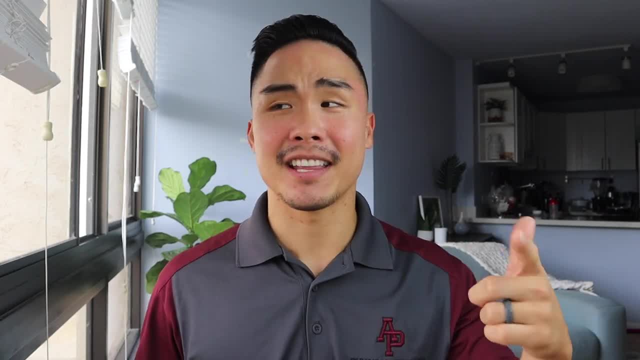 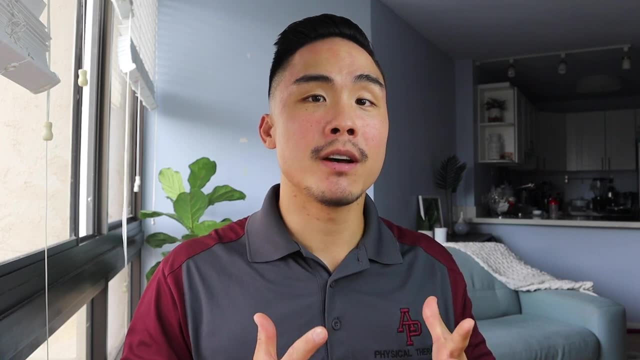 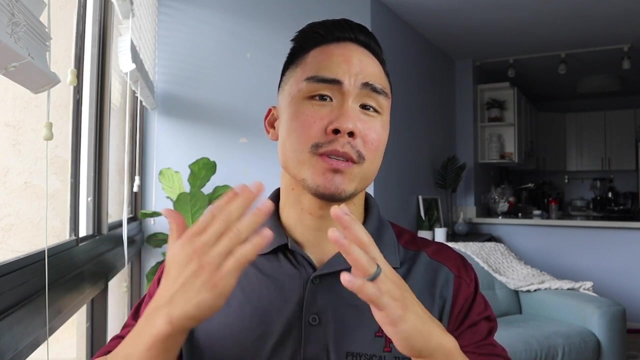 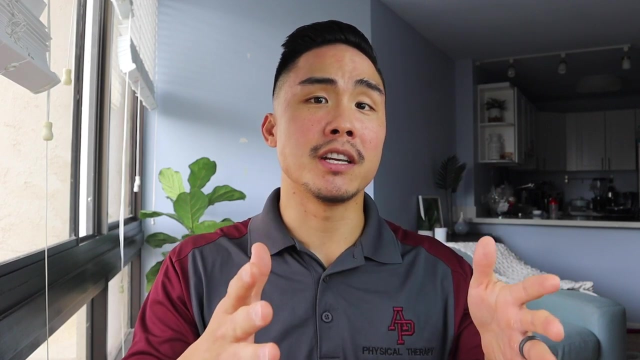 occupational therapists and physical therapy assistants and different fitness professions, right. so to me, That's what I was super passionate about, and I was super passionate about not using Surgery medicine or shots to help someone get feel better, But I was more on the path of conservative care, where I literally used the body to heal itself. 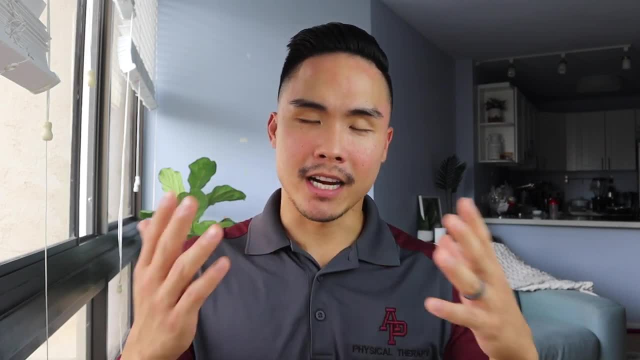 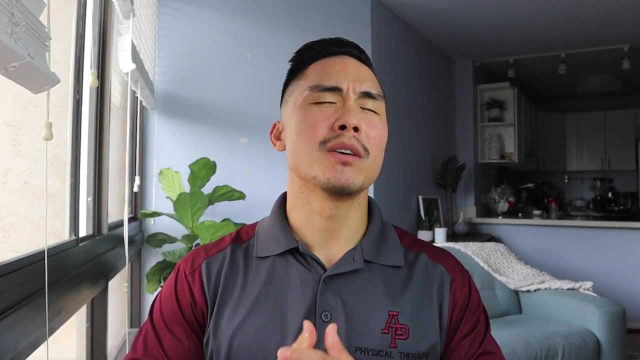 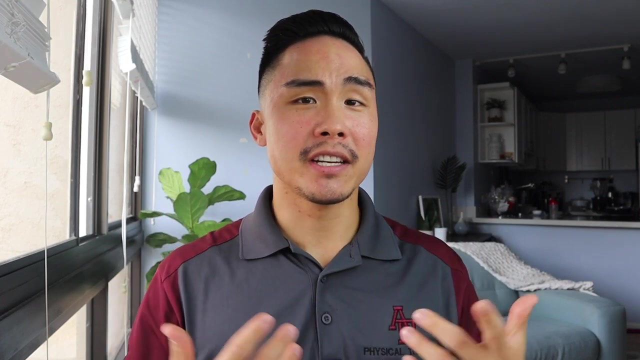 So that's why I chose PT, But, like I mentioned, the amount of money, the cost of schooling and the amount of schooling that you need, Man, PA would be the great, would be a great way to go you. So I hope this video helped inspire you to make an educated guess between either PA or 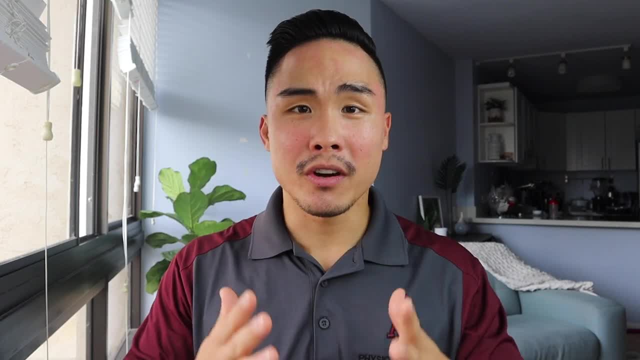 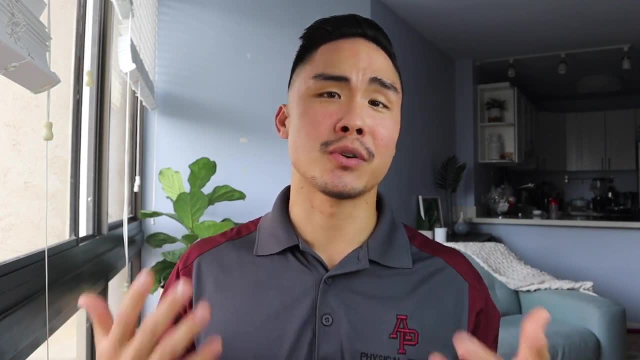 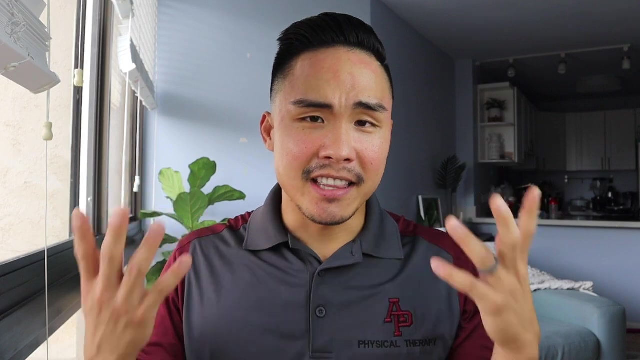 PT, and that you can choose a career and start today to work towards that profession, especially in this time of uncertainty during the pandemic. Now, I truly believe that healthcare- one of the benefits of healthcare is That there is always a stable market for it- Is that there is always a stable market for it. 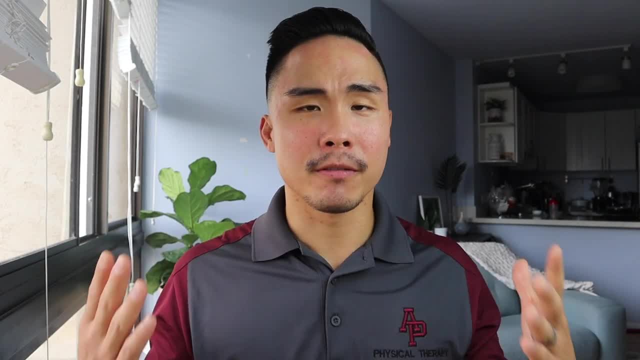 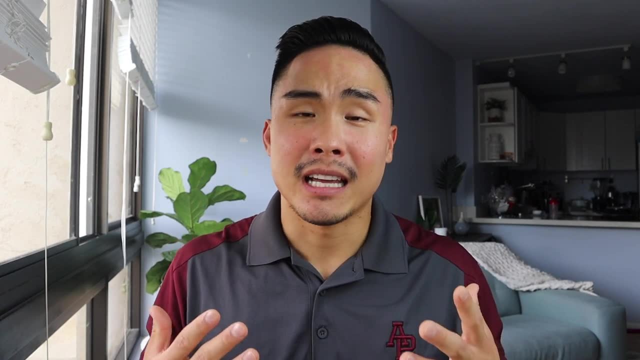 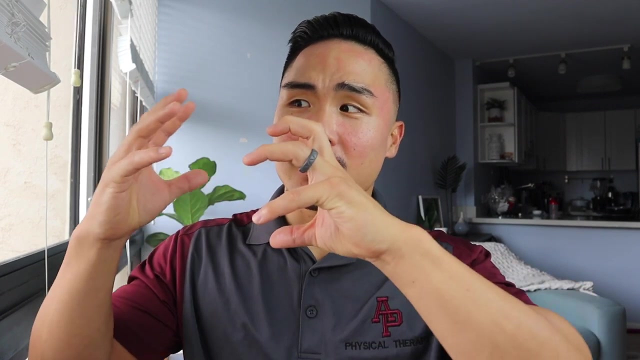 there's: whether any profession you get into a health care profession, you're always going to have stability and it's always going to be a need for the future. right there's so many people- and i'm sorry if this is you- that got unemployed because of this pandemic, but let this this time.